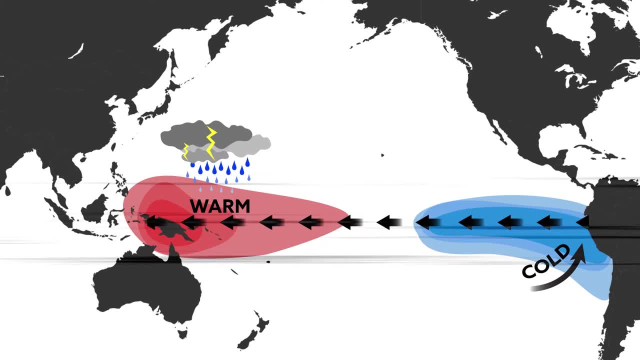 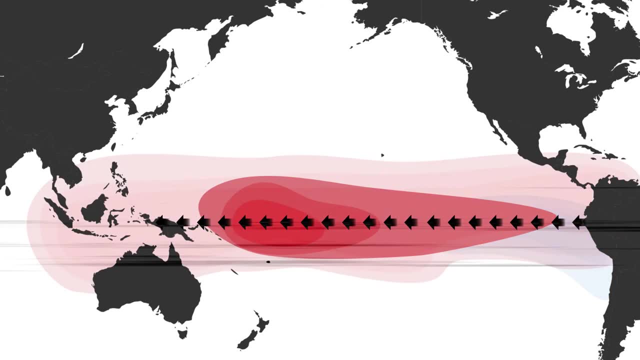 feed moisture into tropical thunderstorms, which help drive global weather patterns. But every few years the trade winds weaken and the warm surface water near Indonesia sloshes eastward, bringing with it tropical thunderstorms and torrential rains. This is the phenomenon known. 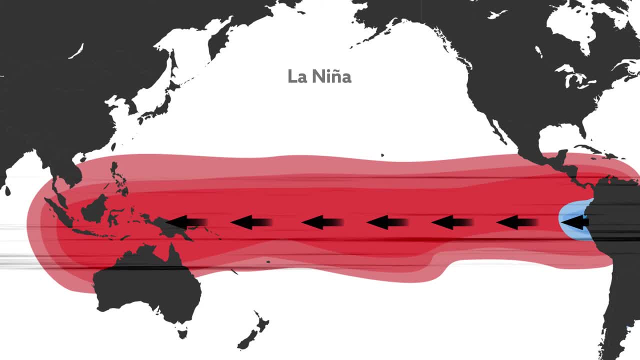 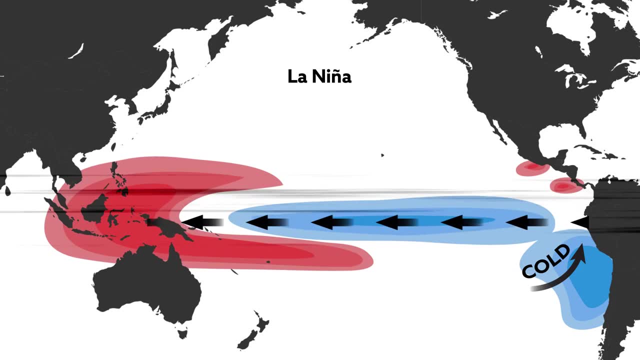 as El Niño. The opposite situation, La Niña, occurs when the trade winds are stronger than normal, boosting the upwelling of cold water in the equatorial Pacific and pushing the warm water and thunderstorms even farther west. These Pacific temperature variations have far-reaching impacts on global weather. 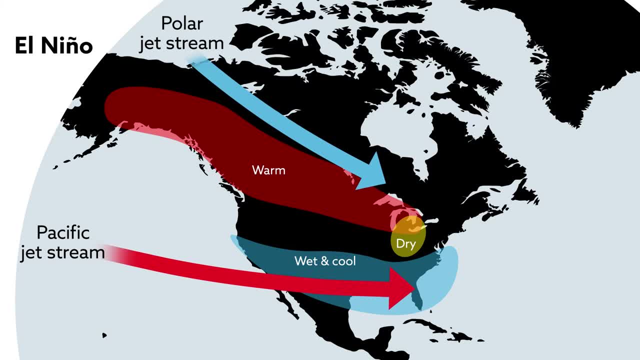 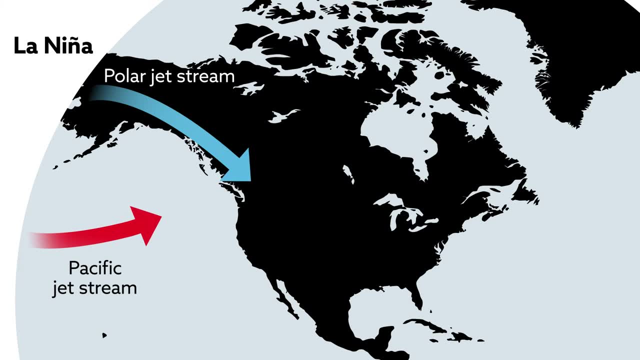 including the likelihood of tornado outbreaks over the US. Using climate data collected over the past 60 years, a research team discovered that both the timing of US tornado outbreaks and the regions where they are likely to occur could be related to El Niño and La Niña. The scientists focused on four different 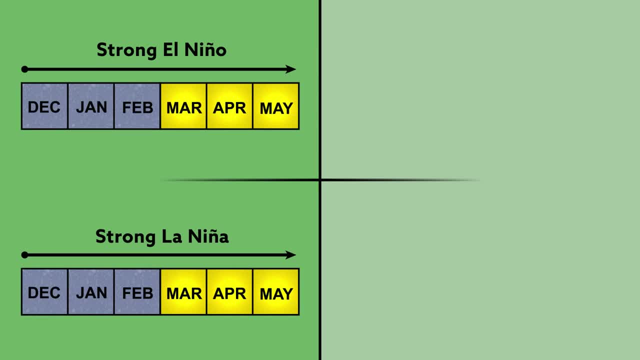 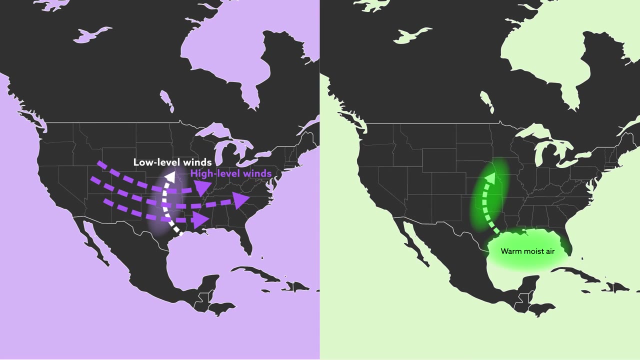 types of El Niño and La Niña events: Strong winter events that persist well into spring and weak events that dissipate soon after their winter peak. The patterns that developed were distinct and consistent with the atmospheric conditions conducive to tornado outbreaks, such as increased wind, shear and the convergence of warm and moist. 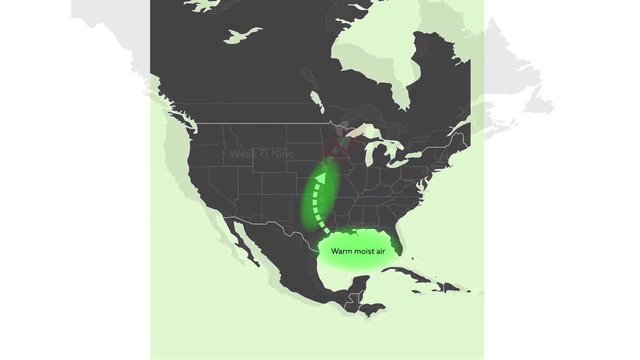 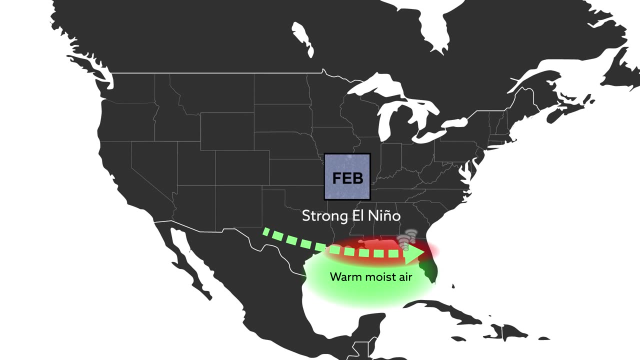 air originating from the Gulf of Mexico. They found that weak El Niños led to tornado outbreaks in May throughout the upper Midwest, while strong El Niños led to outbreaks in February across central Florida and the Gulf Coast. In contrast, weak La Niñas led to April outbreaks throughout. 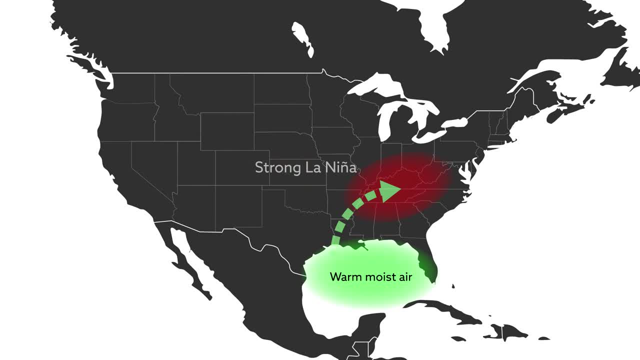 the South, particularly Oklahoma and Kansas. while strong La Niñas led to April outbreaks along the Ohio Valley and in the Southeast and Upper Midwest, The strongest connection to tornado activity was through strong, persistent La Niñas, consistent with the Super Outbreak of 1974 and the record-shattering outbreaks of 2011,, both of which occurred during strong 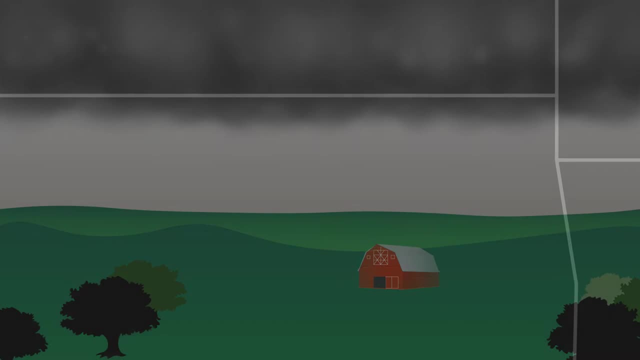 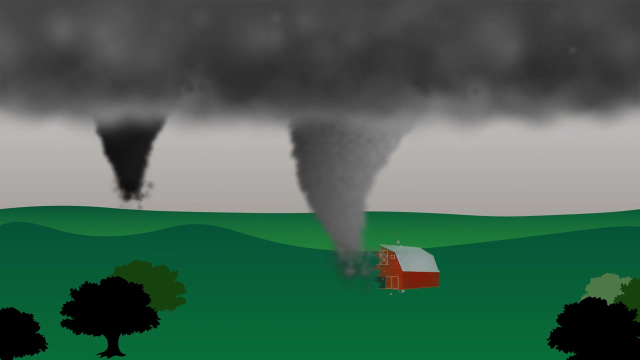 La Niñas. Despite these connections, there is still a large element of chance. An outbreak can occur in any season and almost anywhere in the US, regardless of the state of El Niño or La Niña. The researchers' current work is aimed at